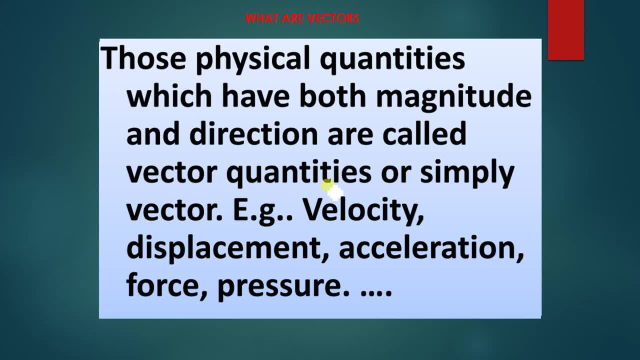 talking about. when you begin to look at the vectors in details, All right, so displacement has magnitude, acceleration has magnitude, force has magnitude and direction, and pressure has magnitude and direction. So these examples of vectors. but when we talk about a scalar? so a scalar only has magnitude but no direction. 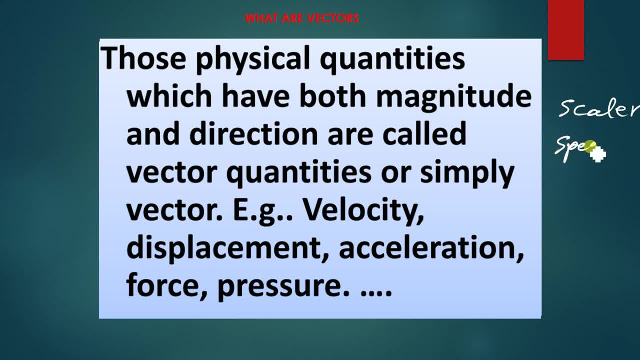 Look at speed: Speed only has magnitude, It has no direction. And when you look at the temperature, temperature also only has magnitude, it has no direction, Can't say this is 35 degrees, 35 degrees Celsius, about a 45 degree celsius year. 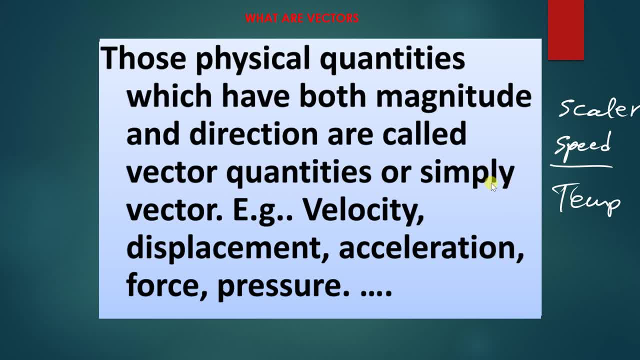 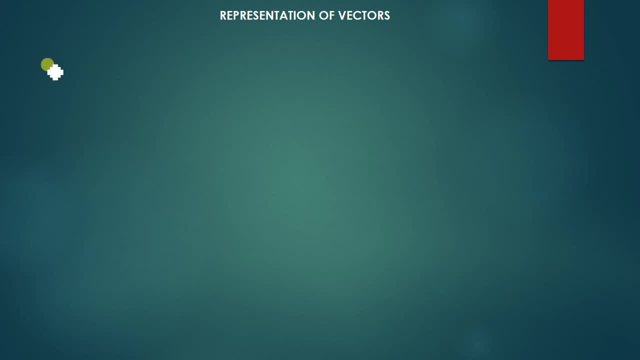 as north. you've never heard about that, right? yeah, so that tells you to say it only has magnitude but no direction. all right, so let's look at how we can represent vectors. so a vector um, a vector can be represented in a, in this form, let's say you have a vector a. so one thing you have to understand if you are 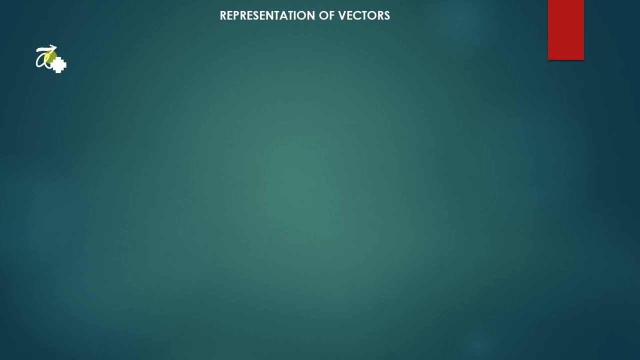 representing a vector, you need to indicate the arrow on top. if you are typing this, a needs to be board, it should be board a. yeah, it shows that it's a vector. and then, if it's not board, then it's a scalar, and then if you can't make it board, then just have to show the arrow on top, then. 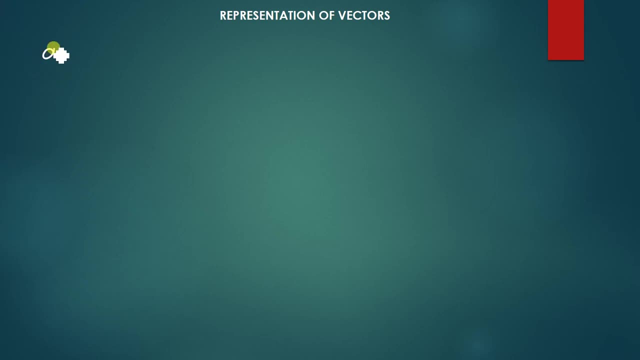 that's how you do it. you represent vectors, and then if you- if, let's say, you have the vector a- yeah, if you have a vector a, uh, being equal to. okay, let me talk about position vectors, if you have the vector a or a. by the way, when we talk about position vectors, these are just vectors. 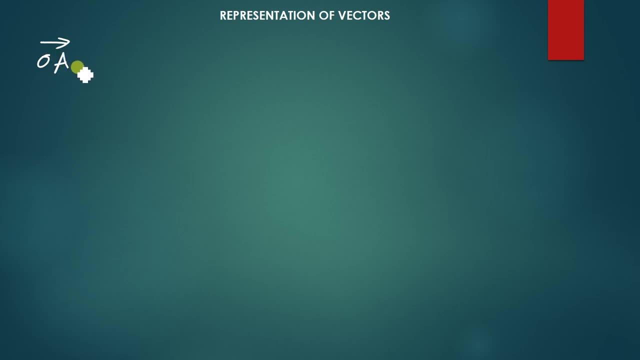 from the same uh origin. yeah, so if we say a and b are from the same origin o, meaning a and b are position vectors. what i mean is this: when you have the vector a and the vector b coming from the same origin o, these are called position vectors. so you can, you can represent this um. 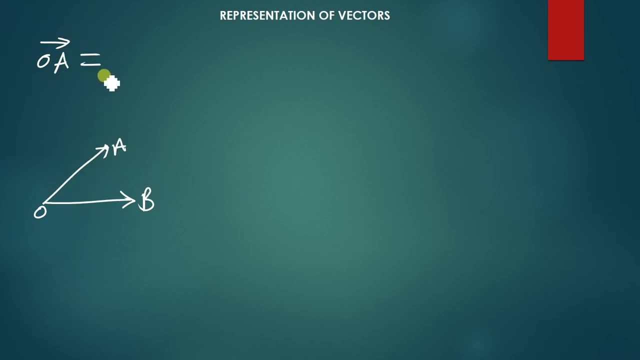 vector a in in in this form, so you can have a, x, i. oh, so sorry, sorry for that. let me do this, you can. you can say a, i plus bj. so if it's in three dimension you add z and k. oh sorry, c and k, yeah. so some books, you find it maybe in this format. let's uh get the other part b. 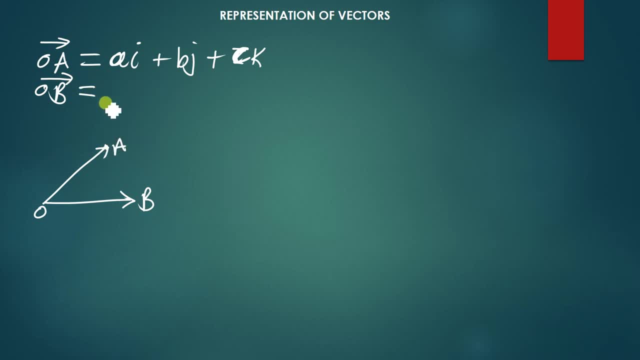 so ob can be represented. so in some books they can't use a and b. they'll use x, uh, y and um z. yeah, so this, this is what um they use in some books. all right, so this is how you can. this is one way of representing vectors. this is known as the cartesian format. 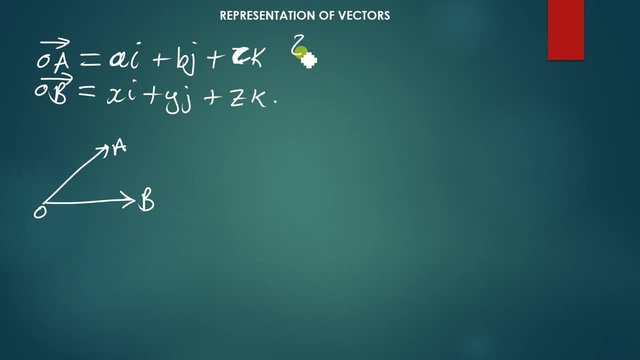 yeah, so this is known as the cartesian format of representing vectors. then you also have another way of representing this same vector, so you can present it as: so you can represent this oa, as you use this type of brackets as a, comma b, comma c, you can also. 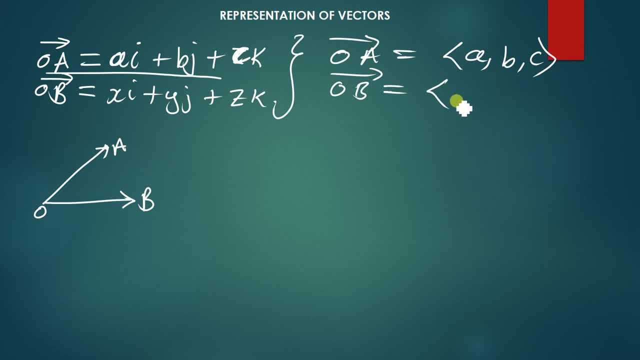 represent b or b as um. x, comma, y comma, z. sorry, this has to be like this. so the moment you just use um, the moment you you just use this type of brackets- they are called parentheses. so the moment you just use um, you just say oa is equal to um. you use this. okay, let me not even say oa, I'll just put. 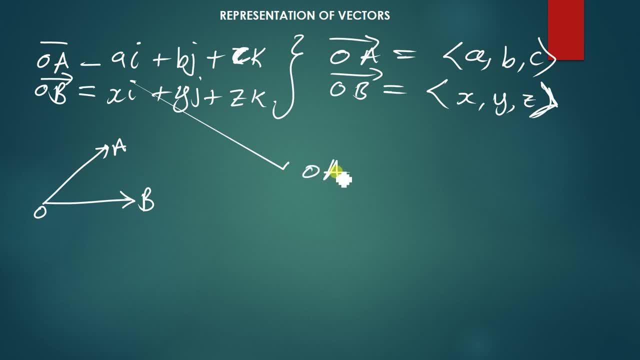 it as yeah, so saying sorry for making it so. how many terms is these? okay, let me just correct it. okay. yeah, I just want to say that I'm closing in on the icon, in this case trigonometric convergencies. where is the私耶��? 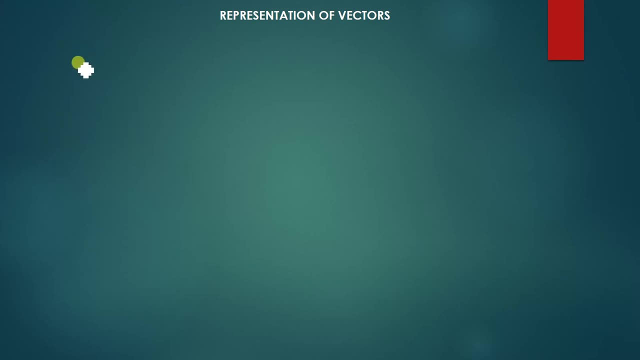 and and and for that. um, if you have oa, you have oa being equal to- i'll just write one: you have oa as a vector and it's equal to uh ai plus bj plus ck. so if you have this as your vector, this is called cartesian presentation of vector. and then, um, you can also present this vector in this notation. 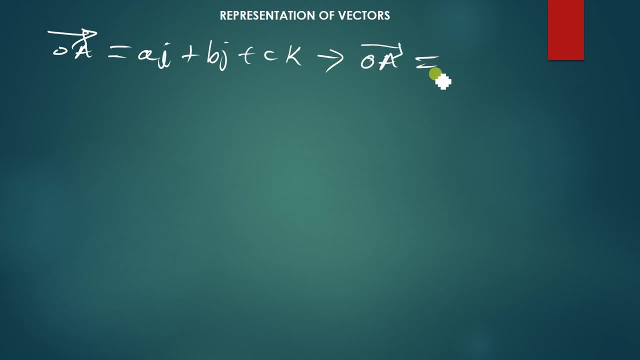 so oa can also be written as a comma b, comma c using these kinds of brackets. so the moment you represent oa as uh, i mean in this format- you use uh parentheses, you say a comma. okay, let me just say, let me not even call it oa. let me just say, if you have anything that looks like this, you say maybe this is uh p. 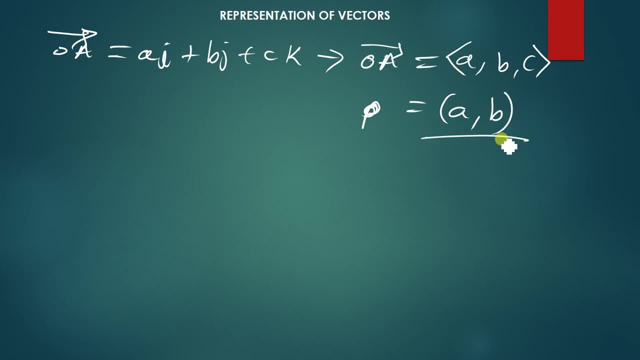 if you have anything that that looks like this, this, this one is called a point. it's a point in space. if you have the x oi plane, if you have the x oi plane like this, you have one, two, three, one, two, three. so if you have this point, 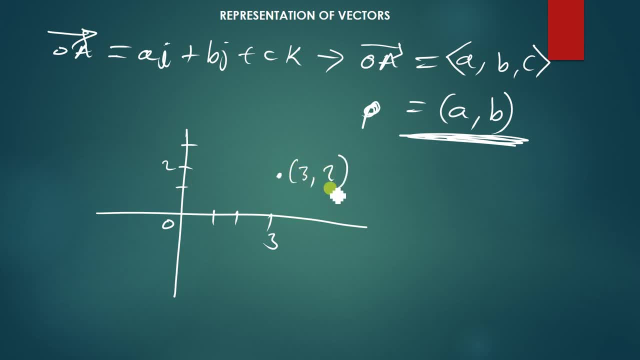 which is 3 comma 2. use parenthesis to represent the point. yeah, so if this is a vector, we change the brackets. so if we change the brackets, we use these brackets, meaning it becomes a vector, which implies that we can even draw it like that. this is what it means. so the moment you just change the types of 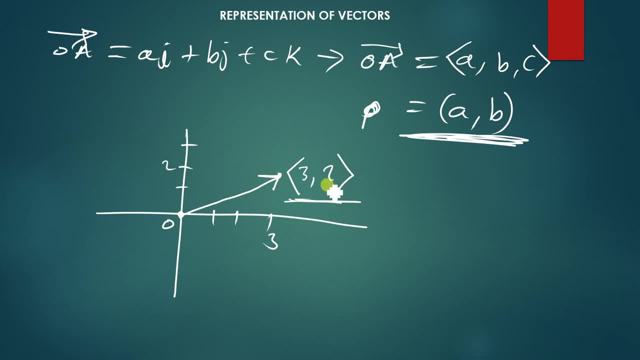 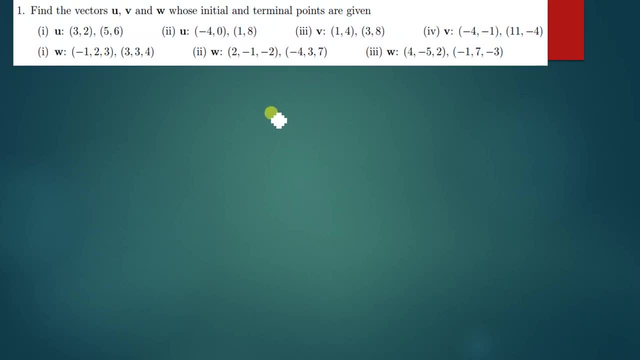 brackets there, the type of brackets there it becomes a vector. all right, so let's quickly look at some examples. so we have this example here which says: find the vector u, v and w whose initial and terminal points are given. so if you have been given the vector a, I mean if you have been given the point a and 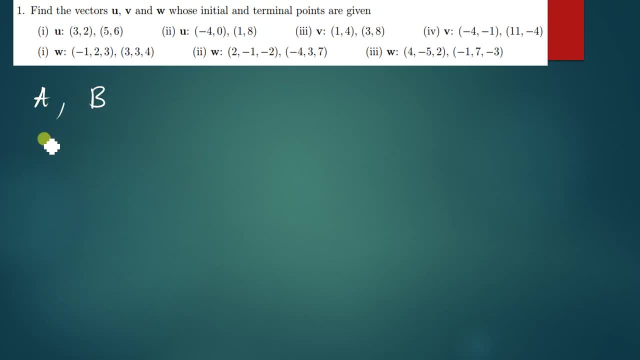 point B and then you've been asked to find the vector a b. you've been given the point a and point b and then you've been asked to find the vector a b. vector a b. if you have. this is point a and point b. now we are asking. 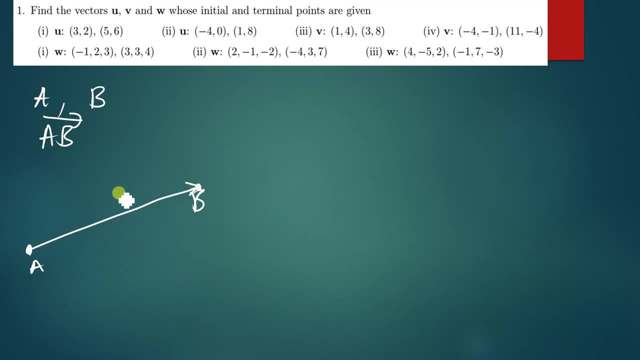 you to find the vector of these two points, or the vector connecting these two points, you simply just subtract the tail from the head. in other words, I'm trying to say you say that the the head minus the tail, so you say b minus a. so b minus a will give you the. 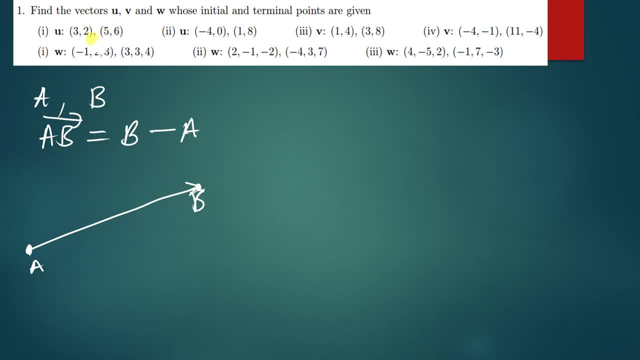 vector a, b. so in this case, if you have these points, like I explained I said, if you are- you- I mean the moment you just see parentheses- you know that what you've been given are points and not vectors. so you've been given points here. you've been given points and you've been asked to find the vectors. 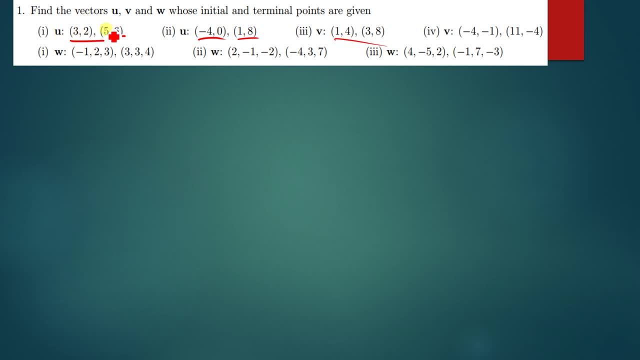 so now let us find the vectors of these two point, these given points. all right, so the first point that we've been given there is, I mean, the first vector I've been given has two points, which is three comma two and five comma six. so these are: 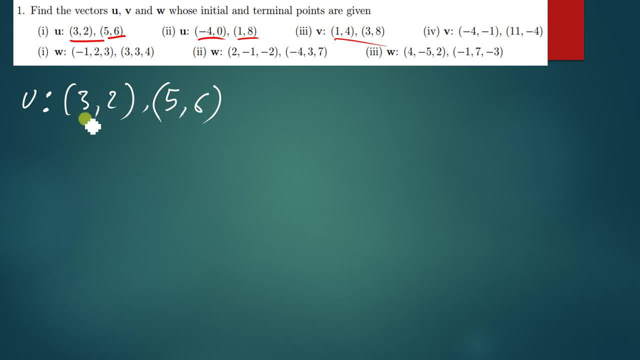 the two points that have been taught to find, I mean used to find- the vector. so our vector you, since we can't make it bold, hence we put a on top. so our vector u is therefore going to be equal to, we say to the head minus the tail. so if 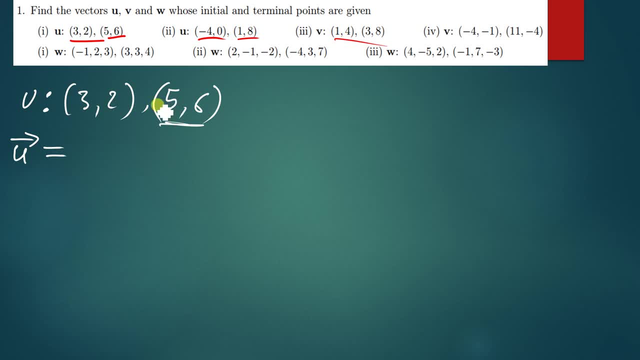 this is our head um, if this is our head um, we say this minus that to find the vector. so i'm going to say, if i want, i can put the points here. i'm going to say five comma six, uh, minus three comma two. so now we can subtract the corresponding um points there. so we have five there. so i'm going to say: 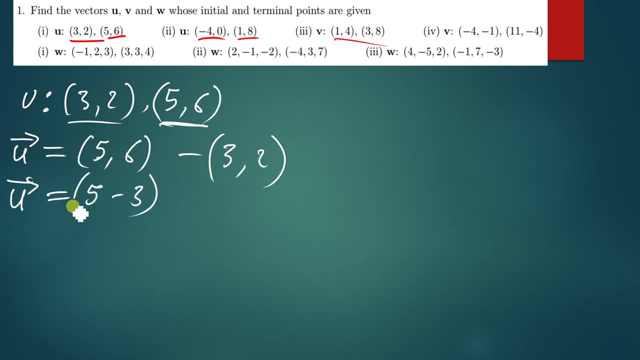 five minus uh, three. in brackets we say comma, so this is now going to become a vector. so let me do it this way. so i'm going to open these types of brackets and then i'll say five minus three, five minus um minus three, so then comma, we will have six. oh sorry, okay, yeah, six minus two. yes, so six minus two. 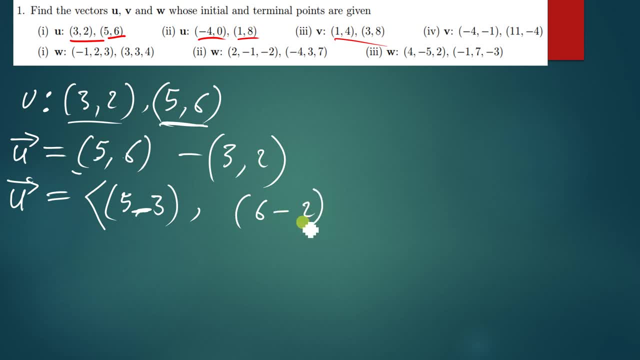 six minus two. so we find the final solution there. so the final solution would be um two comma four. so this is the final solution. so this is the vector u. so we move on to the next uh vector. there we have u, so u will therefore also be equal to. we start with one there, so we 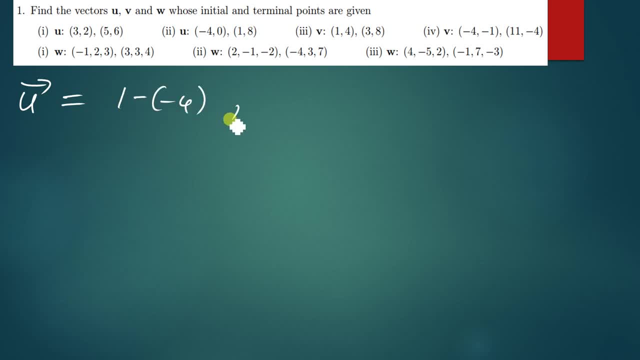 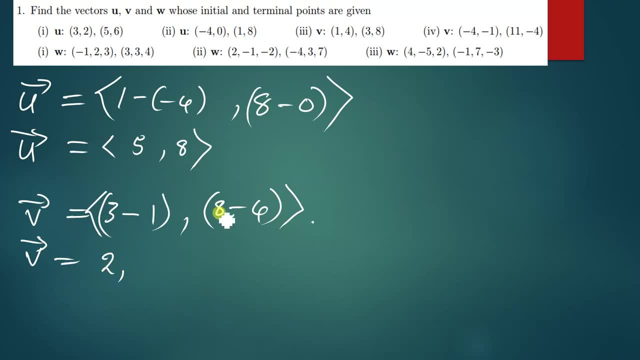 you're going to say 2 comma 8 minus 4, this would be 4. so this is what you get on the solution. so we move on to the other v there. so the other v is um. so the other vector v will be 11 minus negative 4 comma. 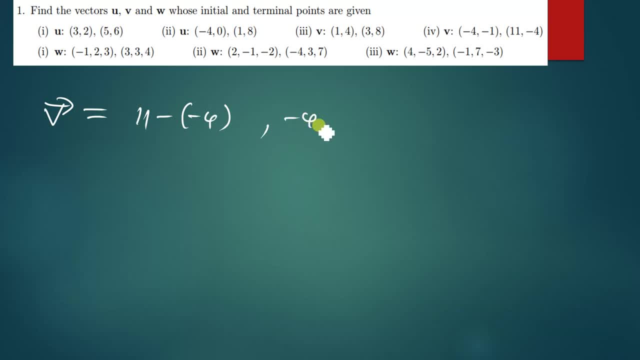 um negative 4 minus negative 1, negative 1. rather okay. so v will therefore be equal to 11 minus 4. there negative and negative will become positive. so 11 plus 4, this will be 15 comma. negative 4 plus 1, because negative and negative will. 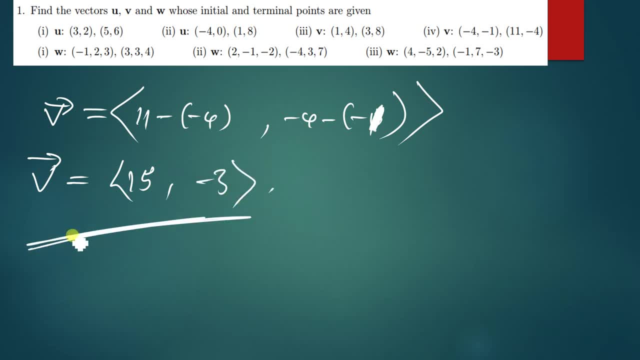 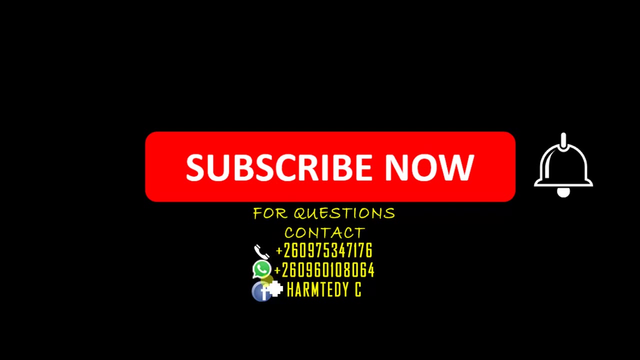 become positive. so we get negative 3 there. so this is our v. let us find our w, so w. i'm going to find one, you find the remaining ones. so if you find the remaining ones, if you want to confirm your answer, you can just simply send it to my uh whatsapp line. you can send it to my whatsapp line. i'll confirm whether. 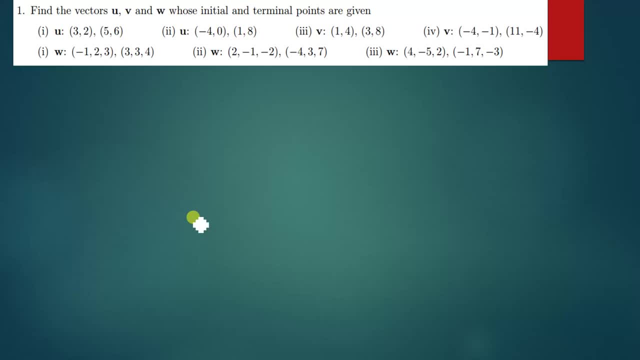 it's correct or wrong, all right, so let's proceed. so w, so for w. we've been given two points there. there is negative 1 comma 2 comma 3 and another point is 3 comma 3 comma 4. so you need to subtract the head from the. i mean the tail from. 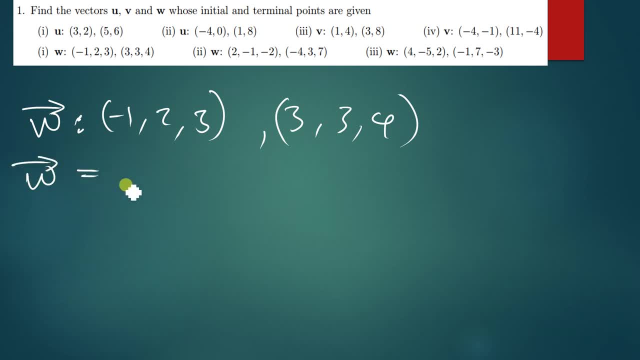 the head. so our vector w is therefore going to be uh 3 minus negative 1, so we say 3 minus negative 1 comma. uh 3 minus 2. 3 minus 2 comma, um 4 minus 3. 4 minus 3. 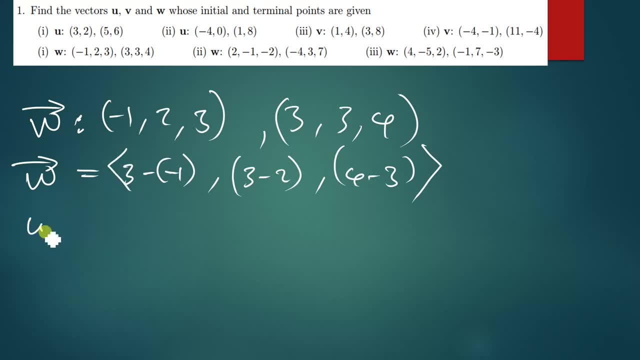 so this is what we have there. so our vector w is therefore going to be 3 plus 1 comma. 3 minus 2 there gives us 1, 4 minus 3. yeah, 4 minus 3 will give us what. 4 minus 3 will give us um 1 again. so 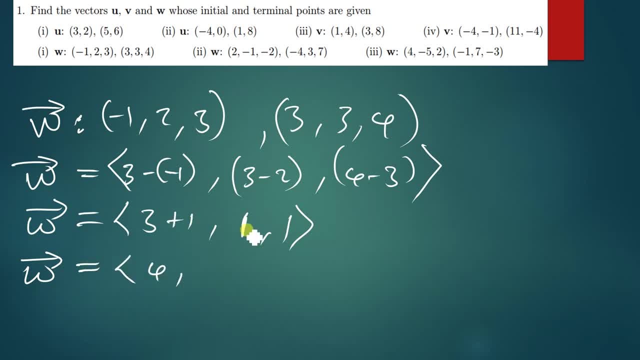 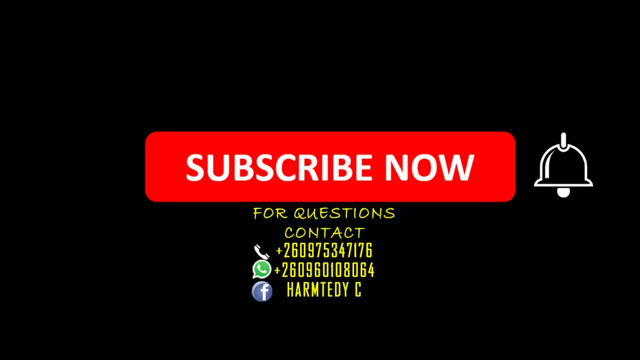 3 plus 1, that will be 4 comma 1 comma 1. so you're going to solve the remaining two questions just to test your understanding. then make sure that you submit your solutions so that i see whether i've understood or not. all right, so feel free to contact me using these lines in case you need lessons in math.